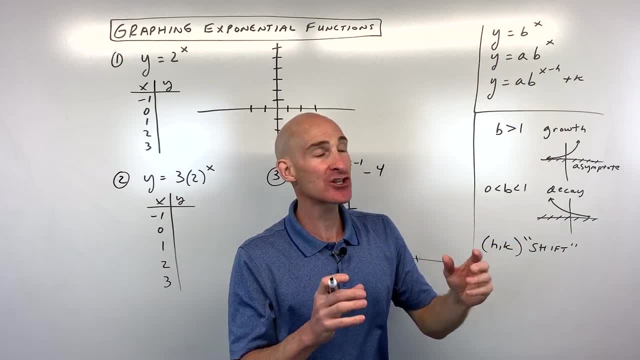 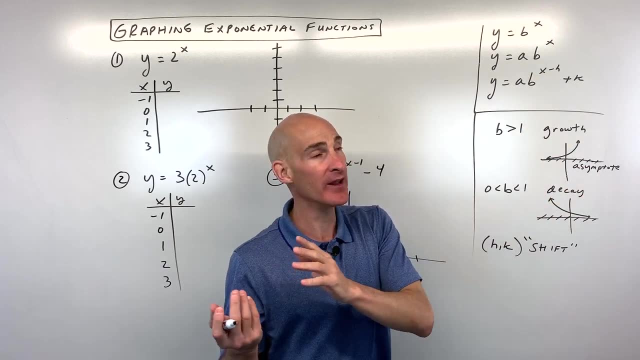 with the x, is going to be shifting it in the opposite direction of the sign. meaning, if this was x minus one, it looks like minus one but you're going to be going right one. If it was plus one, you'd be going left one, Whereas the k value, the vertical shift, if 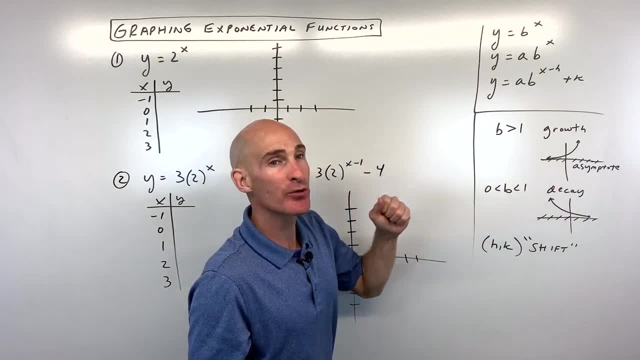 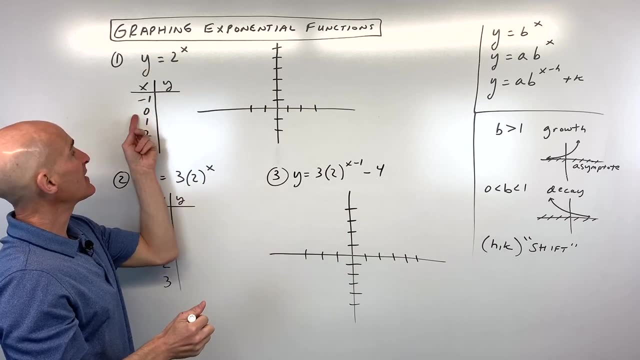 it's plus two, you go up two. if it's minus two, you go down two. So let's go through these five examples. You'll understand as we work through how it works. So a basic one number one, y, equals two to the x. I like to make a table and I pick maybe a couple negative. 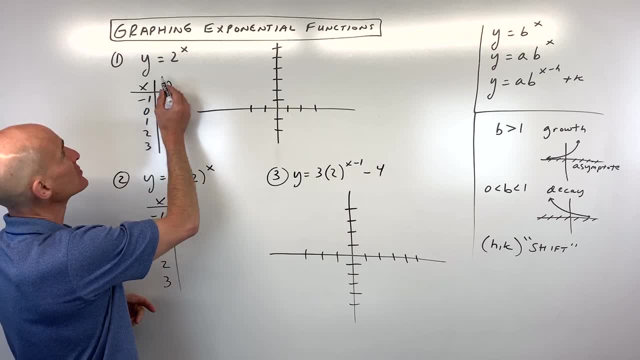 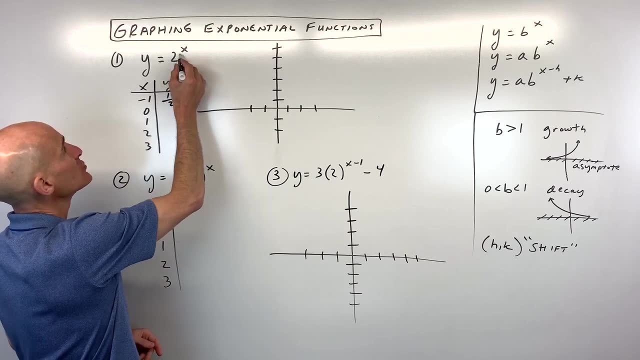 zero and a couple positive, just small numbers, And let's see what we get. So two to the negative, one: when you have a negative exponent you take the reciprocal, so that's really going to be one over two, one half Two to the zero. of course, anything to the zero, power is one. 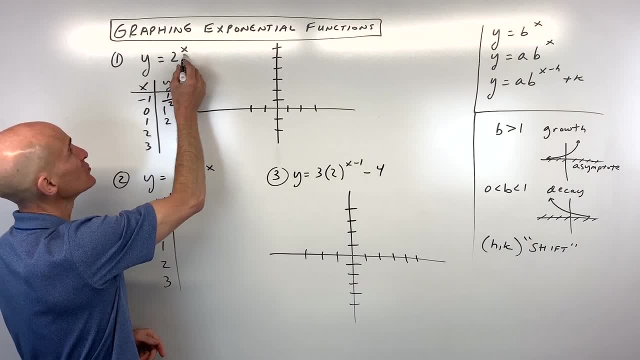 Two to the first, anything to the first, power is itself two. Two squared means two times two, that's four. Two cubed means two times two times two. three times, that's eight. So if we plot these coordinates now, we're going left right, left right, left right. 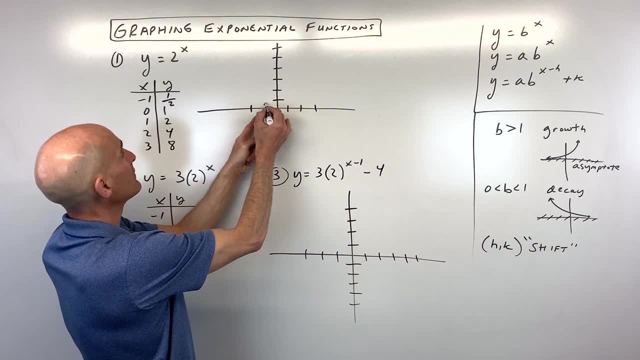 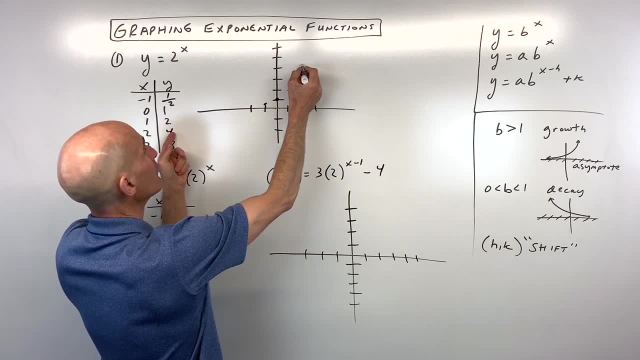 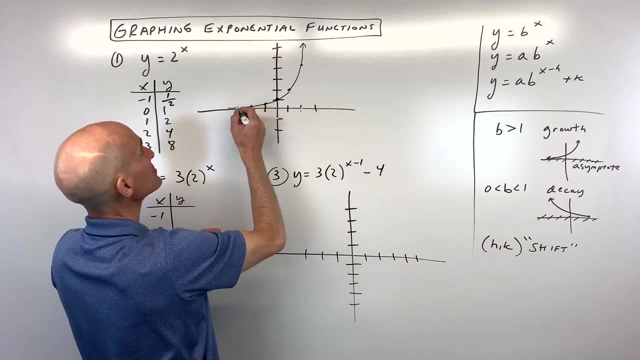 up two, two, four. we're going right- two up four, and then three, eight, right, three up eight, starting to go off the graph. But notice how this is going up faster and faster as we go to the right. that's exponential growth And we knew that because this base was greater. 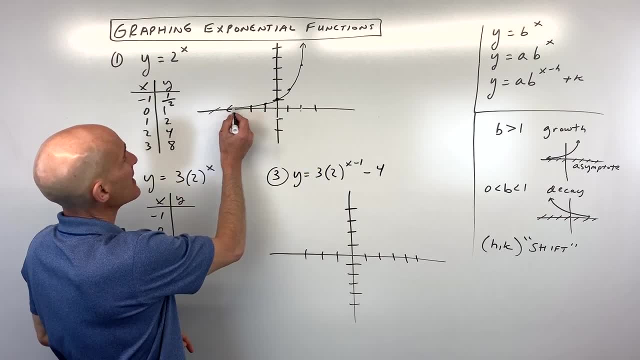 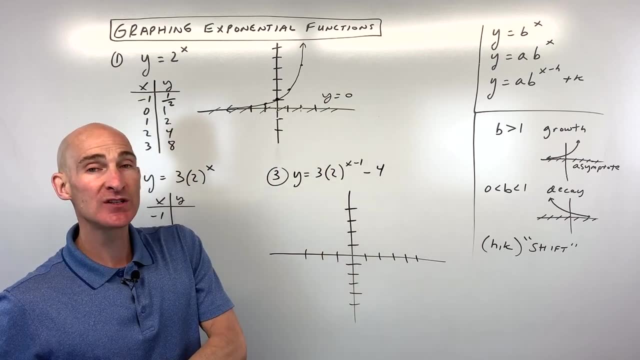 than one. It's getting closer to the asymptote here. the x axis, this is the line y- equals zero, The horizontal asymptote, And often times when you do these problems, your teacher will say: what's the domain and range? Now, when you think about the domain, you say: well, what? 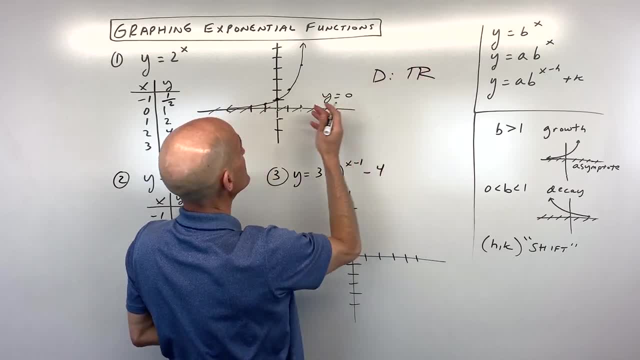 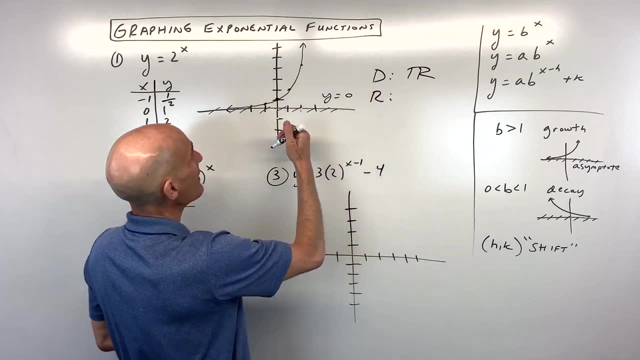 can x be? That's going to be all real numbers. It goes to the left, it goes up, but it's gradually going to the right, forever and ever. So domain x can be all reals. The range, the y values, are just going to be above the x axis. so we say y is greater than, but not. 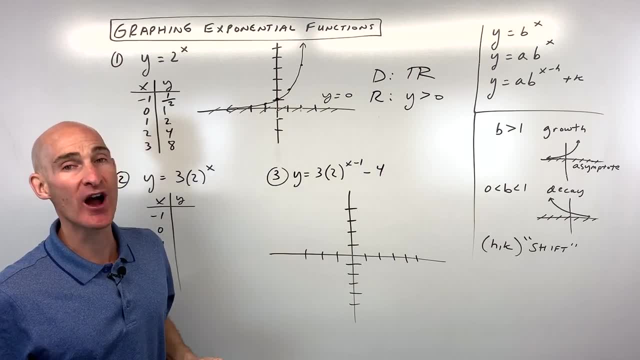 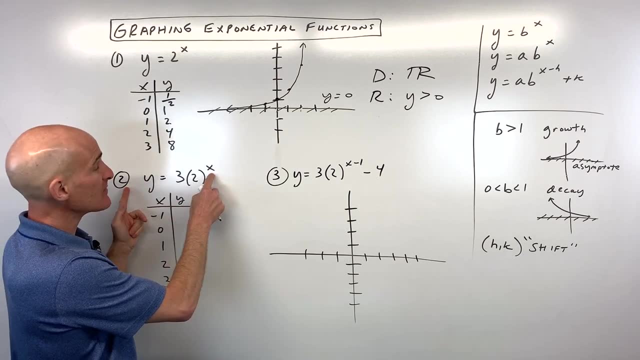 equal to, because it gets closer to this asymptote, but doesn't touch, doesn't cross. Ok, so that's kind of like a basic one. Number two, though: we're building on that. See how we have: y equals three times two to. 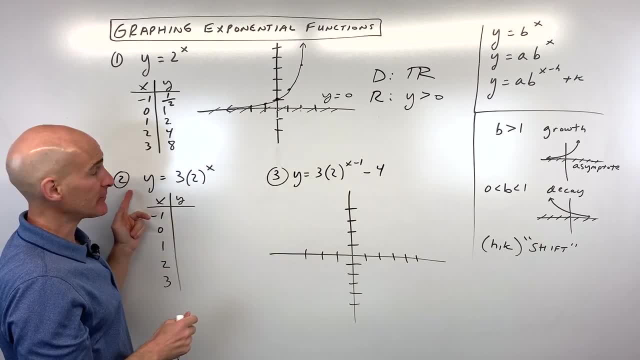 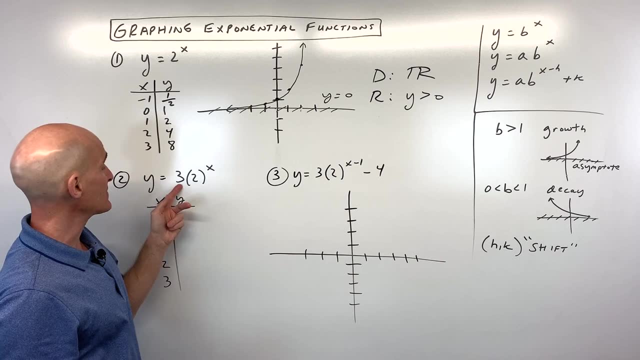 the x. What do you think this three does to this graph? Well, the three, because it's greater than one. it's going to be a vertical stretch. ok, by three times We can go ahead and make a table of values again. And what you're going to want to do- and this is where students 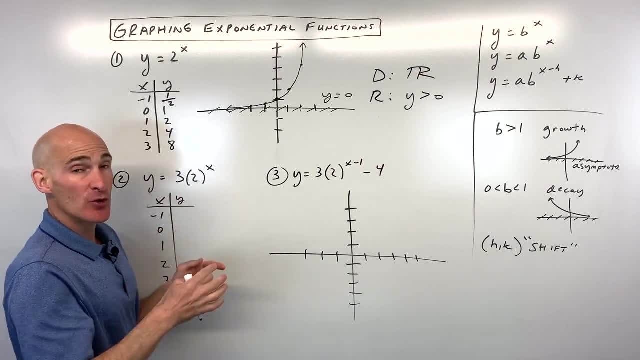 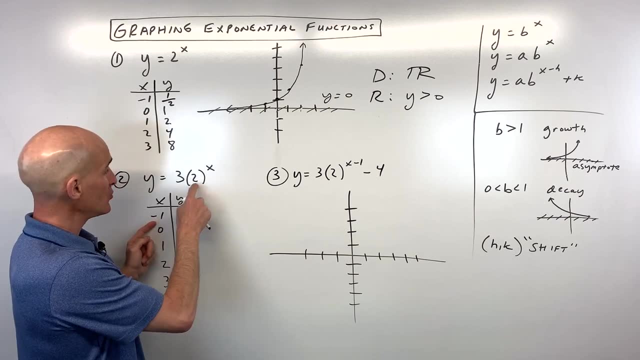 sometimes go off a little bit is. we're used to reading from left to right, but you want to follow the PEMDAS, the order of operations, So you want to do the exponents first and then multiply by three. So two to the negative one we said was one half times three is three halves Two to the 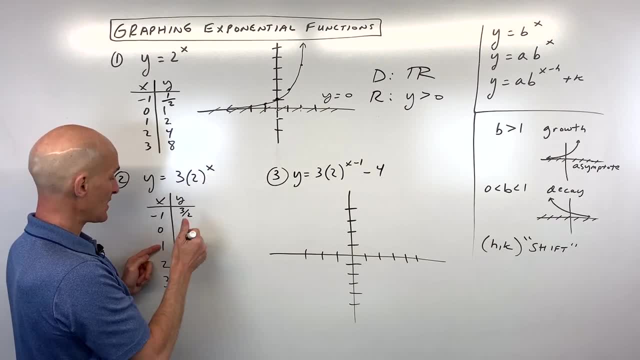 zero is one times three is three. Two to the one is two times three is six. Two squared is four times three is twelve. Two cubed is eight times three is twenty-four. Of course I could have just used these numbers and multiplied by three, but if you were just given this, 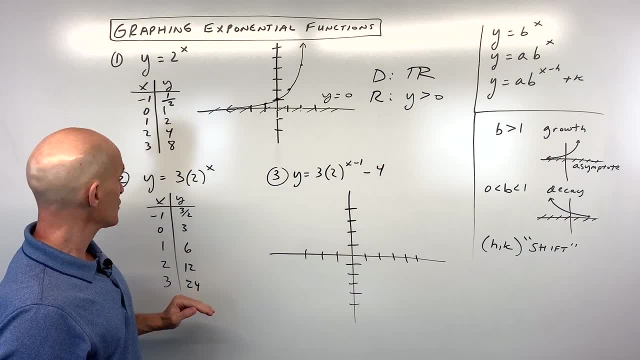 problem, you know. on its own, it's good to know the order. So let's go ahead and graph this on the same graph here. If I go left one, I'm going up three halves, which is one and a half. I'm going up three halves, which is one and a. 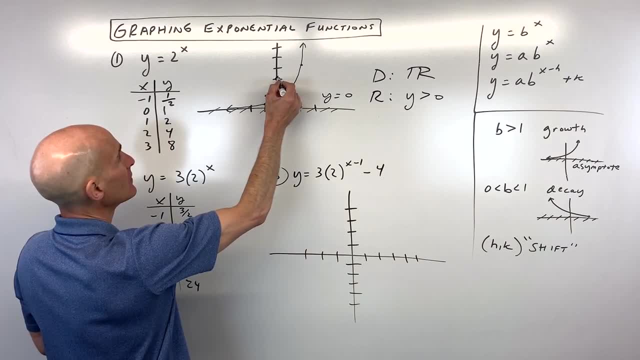 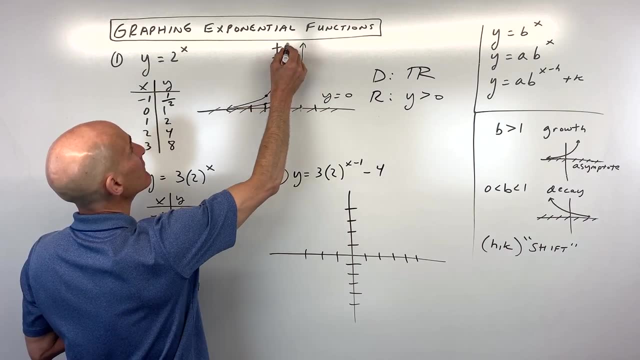 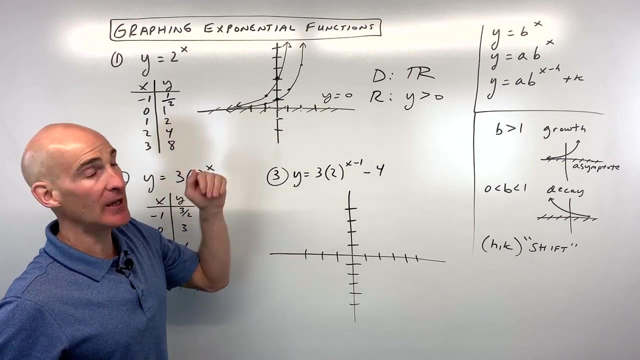 half Zero, three, One, two, three, One, six, Right one up six, And so you can see what's happening. is this graph's like going up like faster, you know, because we're stretching it by three times, It's still approaching the x-axis, okay, and it has the same basic. 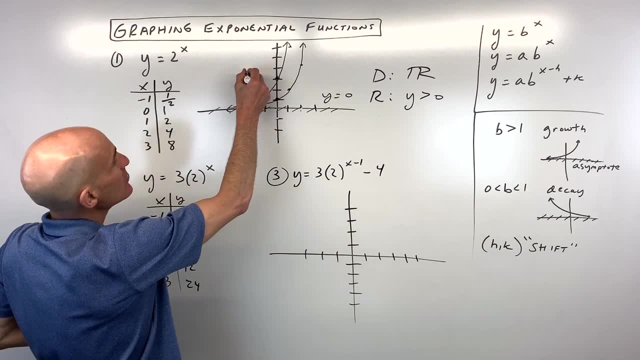 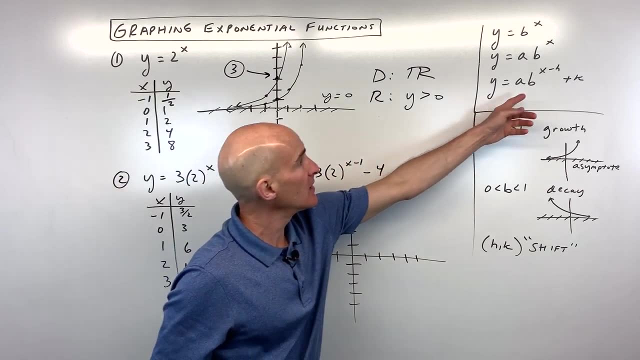 shape. It's just going up quicker, right. One thing you'll notice, though, is you see where it crosses the y-axis, here at three, and notice how the coefficient was three. So if the graph isn't being translated or shifted with this h and k, you can think of this a-value as your y-intercept. 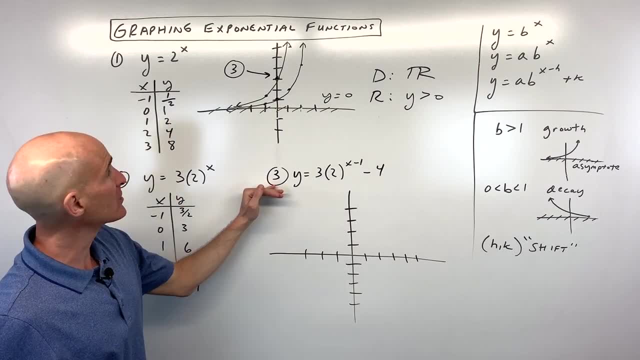 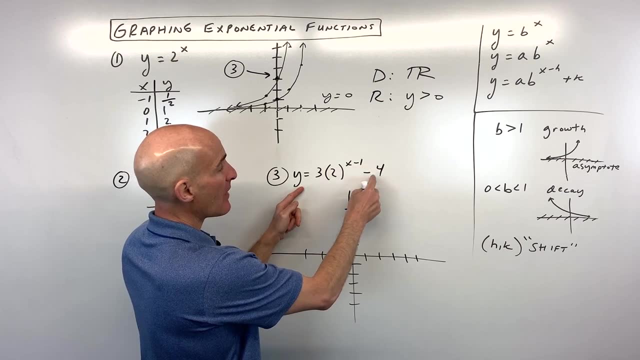 okay, So just a little hint there For number three. now we're taking the same graph one step further. Notice you've got y equals three times two to the x, but now we have minus one and minus four. So what does this minus one do to the graph? Well, remember how we 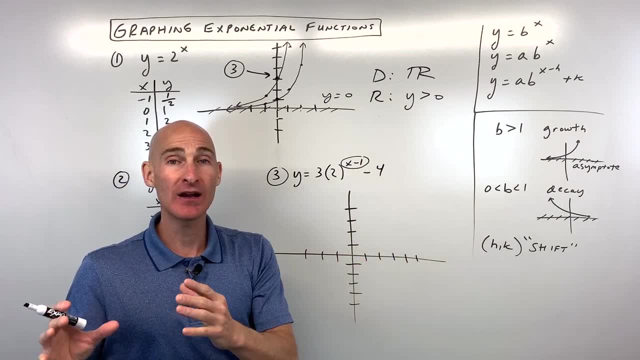 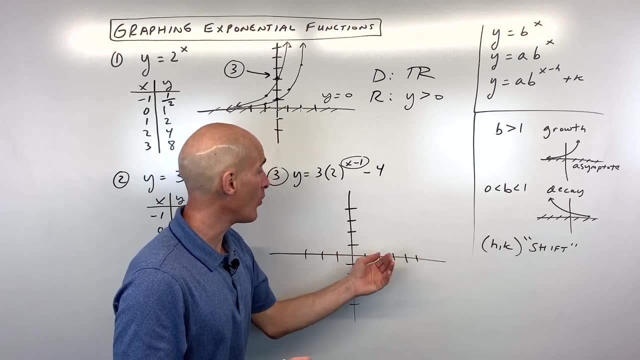 said, the one group with the x shifts it in the x-direction left and right, But it has the opposite effect from this negative one. You would think it would go left, one right, It actually goes right one. This one has the same effect. The minus four is going to go down four. So what I like to do is I like 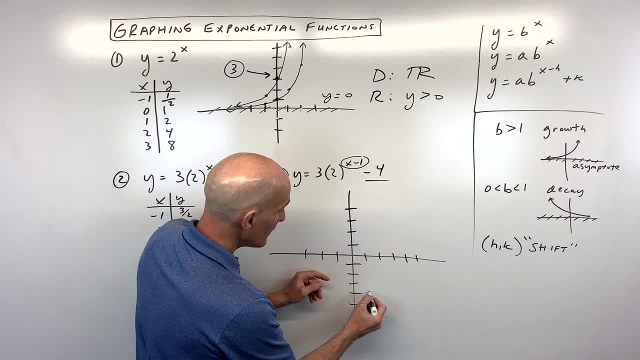 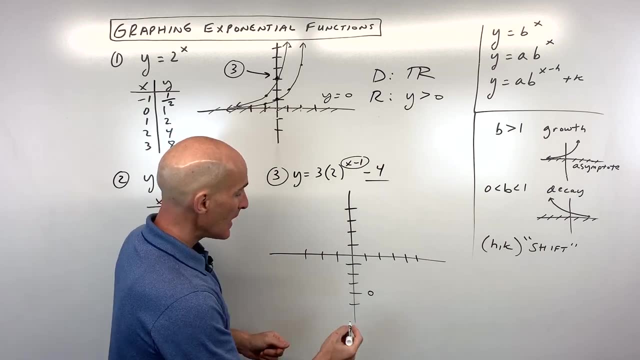 to think of going right one down four, and I put a little open circle like that. What that represents to me is that's like our new starting point, our new origin and, if you want, what I sometimes do is draw in this horizontal line. that's our horizontal asymptote. 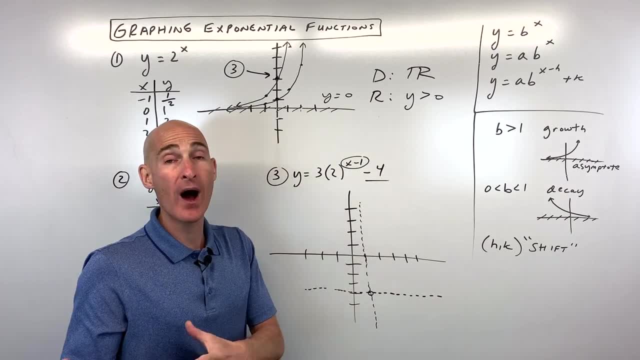 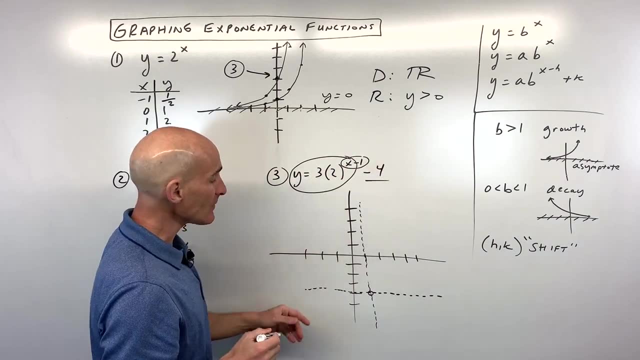 and you can even draw in a vertical line. You can kind of think of that as like your new y-axis. So we've taken care of the translation or the shift. Now we're just focusing in on the parent function. but we're going to be graphing from here, not the origin right, So from 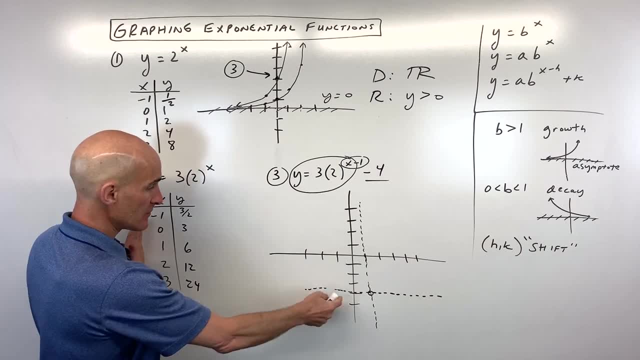 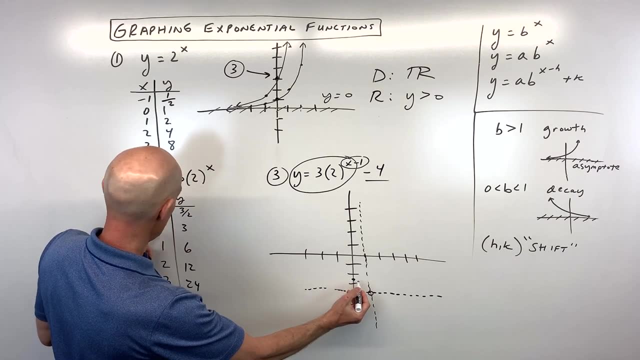 this new origin. We can graph these same set of points from here. So we're going to go left one up three halves. That's going to be right here. We're going to go zero three. so we're not going left to right, just up three, one, two, three, One six. we're going. 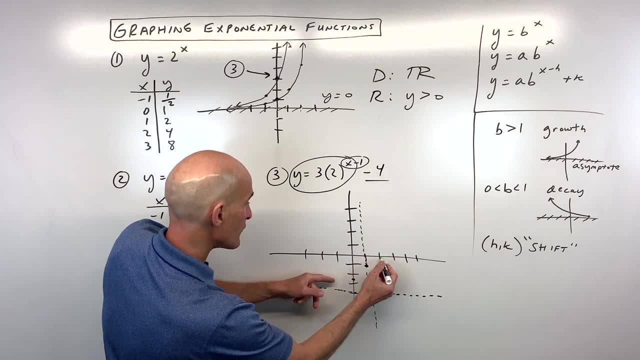 right, one up six. That's going to be, let's see, four, five, six, seven, eight, nine, 12,, 13,, 14,, 15,, 16,, 17,, 18,, 19,, 20,, 21,, 22,, 23,, 24,, 25,, 26,, 27,, 28,, 29,, 30,, 31,, 32,, 33,, 33,. 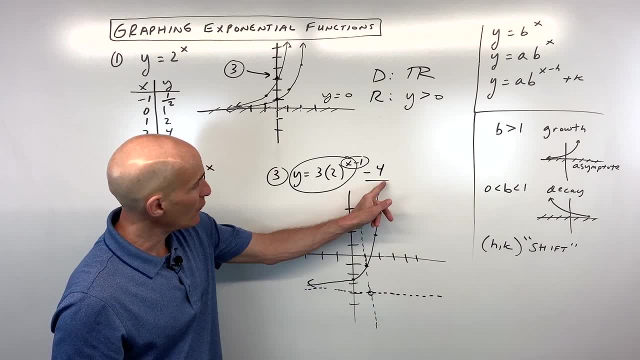 34,, 35,, 46,, 38,39,, 38,, 39,, 40,, 41,, 42,, 43,, 45,, six, And then you can see it's starting to. you know, go up faster and faster is going off of our graph. Now this one because 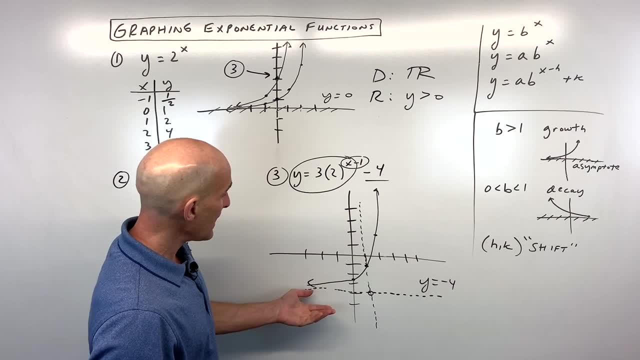 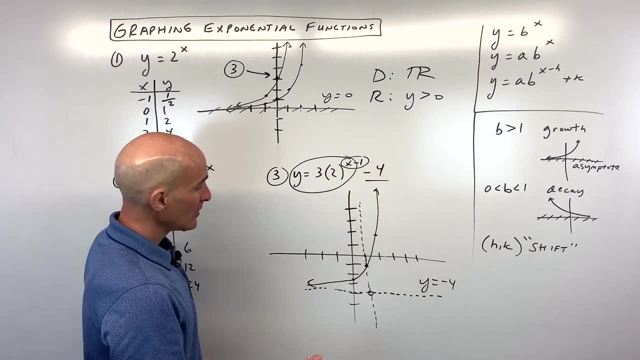 it was shifted down four. this horizontal asymptote right here is going to be y equals negative. four, Remember horizontal lines, or y equals lines, And then the domain is going to be all real numbers. so you'll notice, for these exponential graphs it's always going. 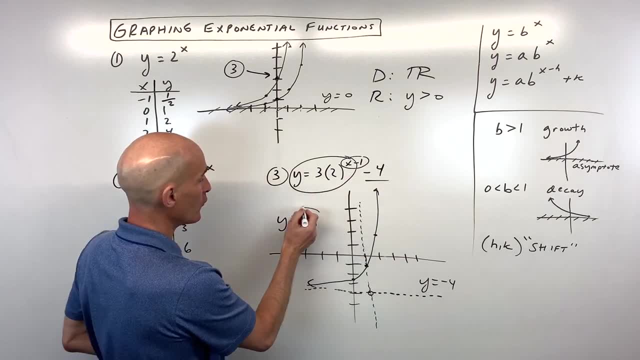 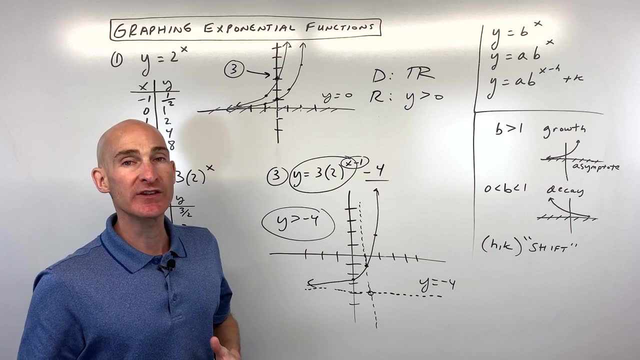 to be all real above negative four. That's your range And you've got it. Let's go through two more examples that are a little bit different than these ones so you can get some more experience. Okay, see if you can do number four and five Really test. 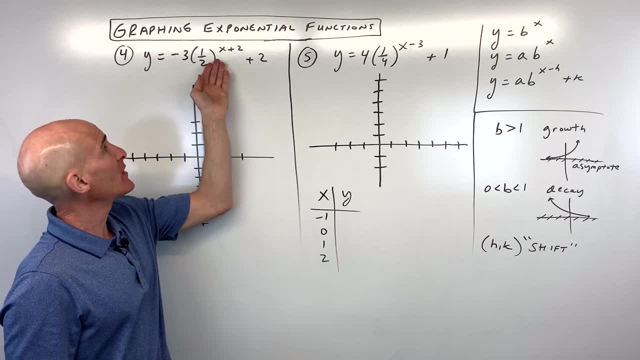 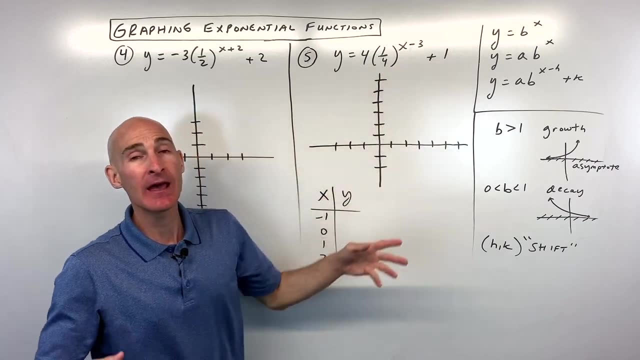 yourself. Graph y equals negative three times one-half to the x plus two plus two. And number five, y equals four times one-fourth to the x minus three plus one. And while you're doing that, I just wanted to introduce myself. My name is. 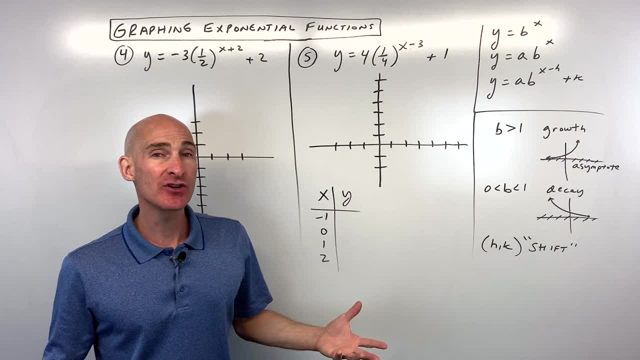 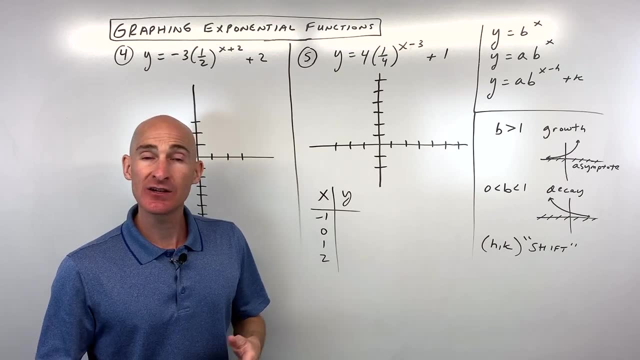 Mario of Mario's Math Tutoring- if we haven't met yet- And my channel is all about making learning math less stressful, so you can raise your grade, pass your class and go on to pursue your dreams. If that's something that's interesting to you, go ahead and check out more videos on my Mario's Math. 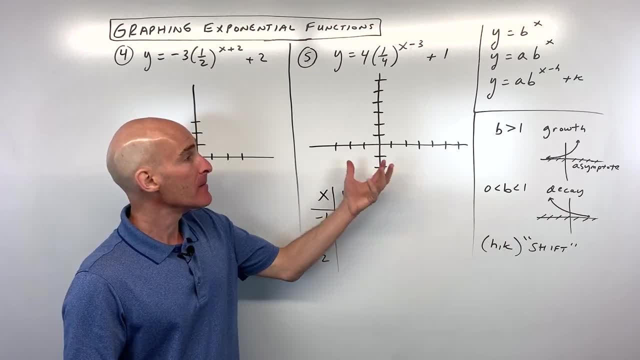 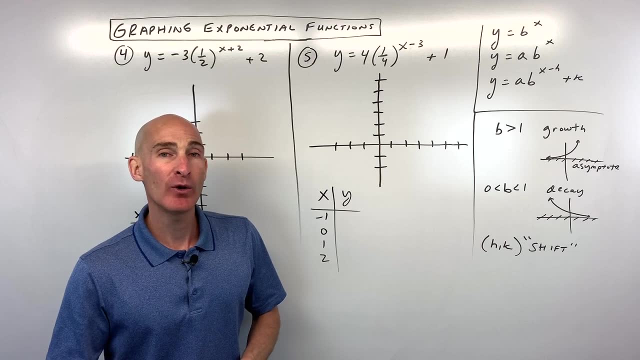 Tutoring YouTube channel, And I also want to let you know that I have math courses, video courses like Algebra I, Algebra II, ACT math, SAT math. That's something that would help you along your math studies. But let's jump into number four here. 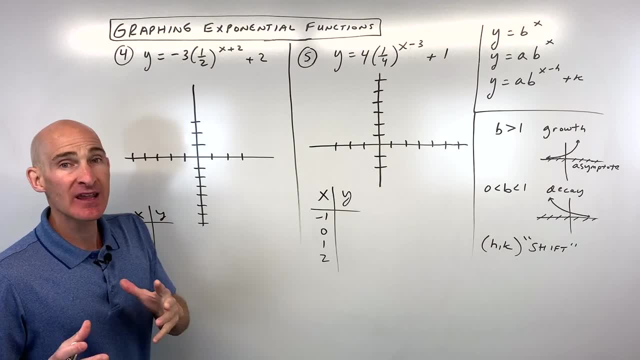 What do I do on this problem? when I look at it, The first thing that I like to do is look at the shift, or the shift in the shift, in the shift in the shift, And I remember the translation And remember this number, that it's a group with the x. 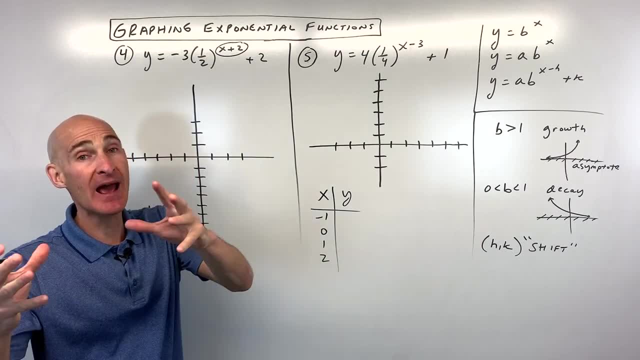 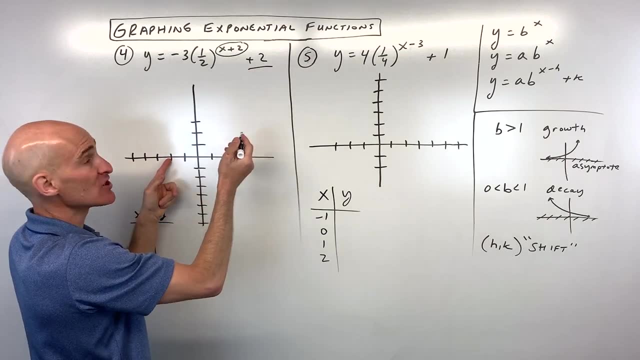 here is shifting the graph in the x direction right, But it has the opposite effect. So plus two means it's actually going left. two: This guy over here is a vertical translation up two if it's positive two. So that means we're gonna. 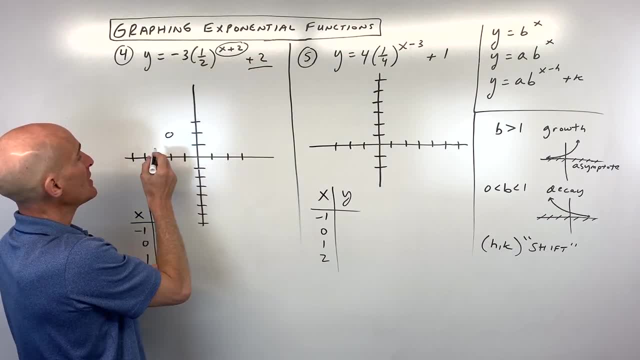 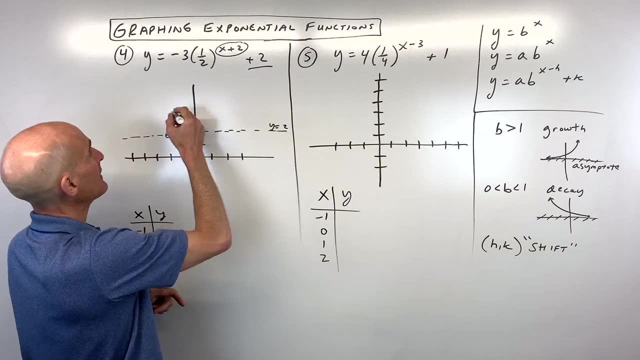 go up two, Just remember, opposite and the same. So then what I like to do is go ahead and draw in my asymptote, okay, which is the line y equals two here, And you can also draw in like a dashed or dotted vertical line You can think of. 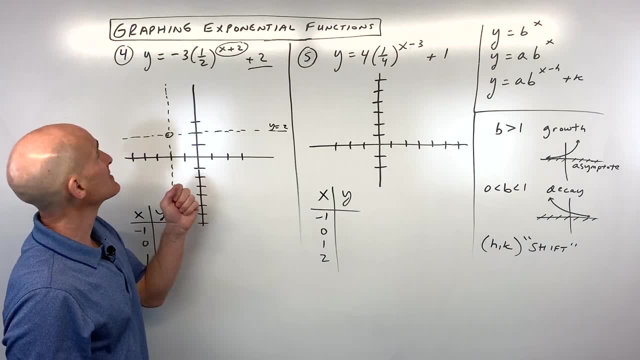 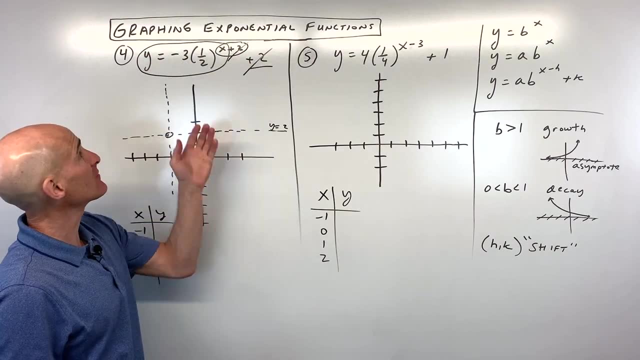 this as, like your new y axis, You don't have to draw that line, but sometimes that's helpful. Then what I like to do is focus in on what's left after I took care of the translation, the shift. This is what I refer to as the parent. 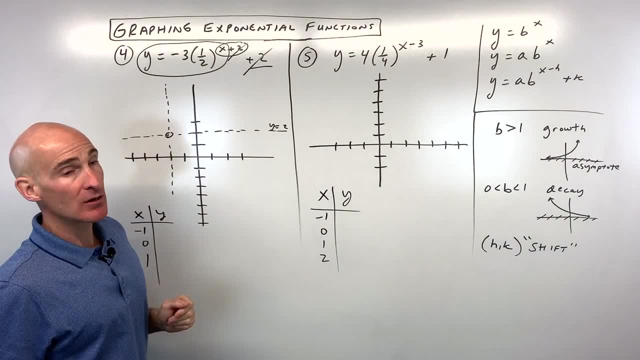 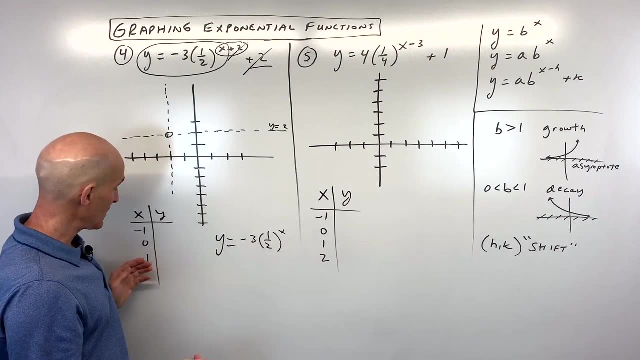 function And I like to make a table just using this equation. So let's go ahead and write that down. Y equals negative three times one half to the x. Pick some simple values. Usually I pick negative 1,, 0,, 1.. If you want some more points, you 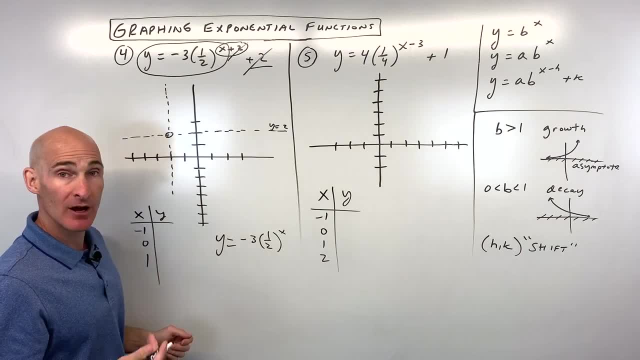 could do negative 2, negative 1, 0, 1, 2.. So a couple negative, a couple positive and zero. If I put a negative 1, one half to the negative, 1 tells us to take the. 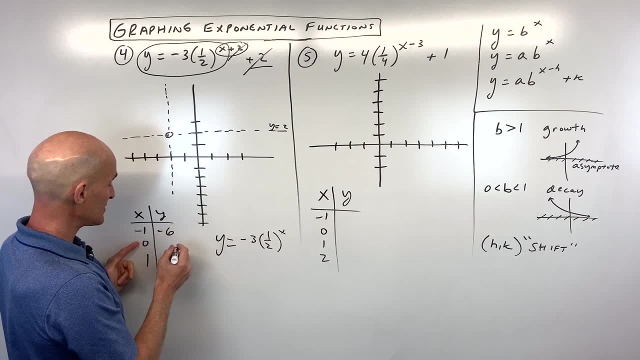 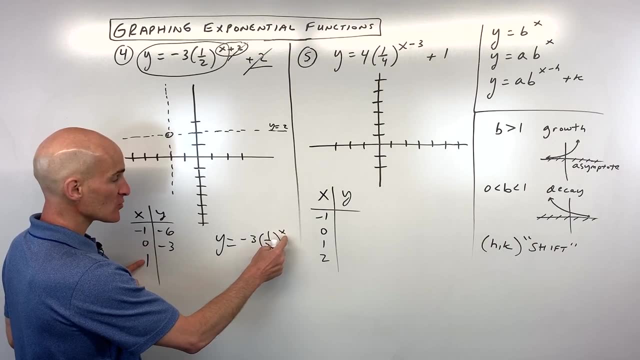 reciprocal. That would make this: 2. Times negative 3 is negative 6. One half to the 0 is 1.. Times negative 3 is negative 3. One half to the 1, first power is one half. Times negative 3 is negative three halves. Now, if we plot these points not 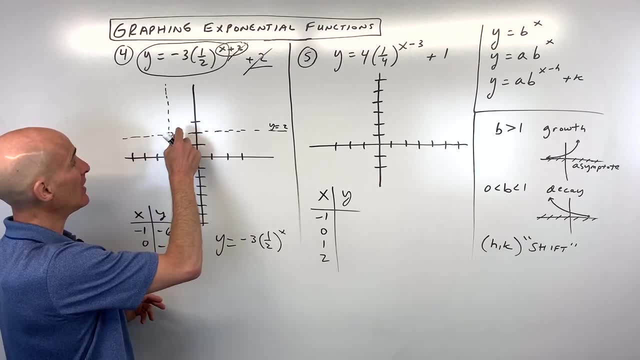 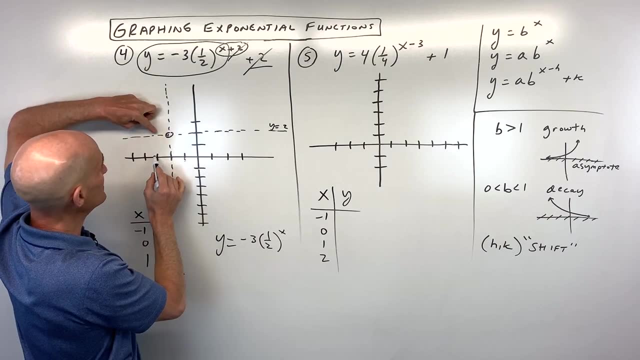 from the origin, but from the shifted origin. the origin, that's where it's been translated. we're going to graph from here. So we're going to go negative 1, negative 6, so left one Down, 6, that's 2, 3,, 4, 5, 6.. Right about there. 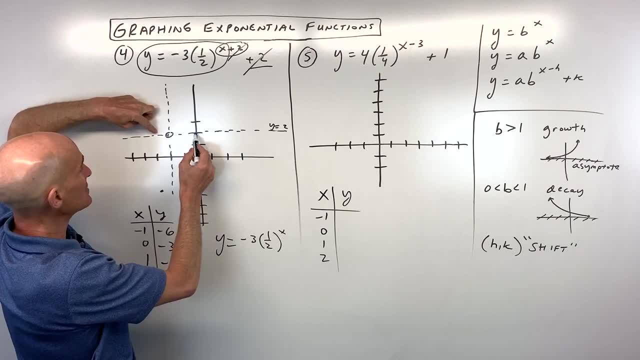 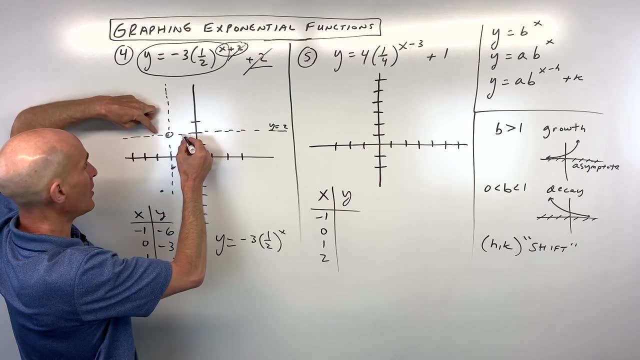 OK, And we've got 0, negative 3.. So this is going to be 0 left to right down 3. It's going to be right about there, And 1, negative 3 halves. So we're going right one. 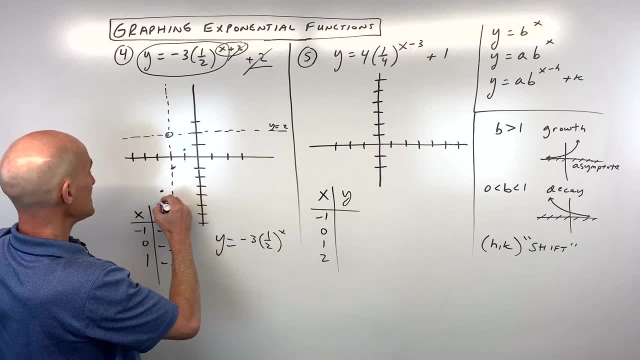 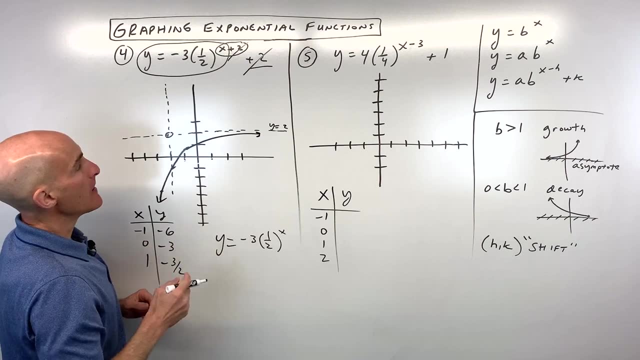 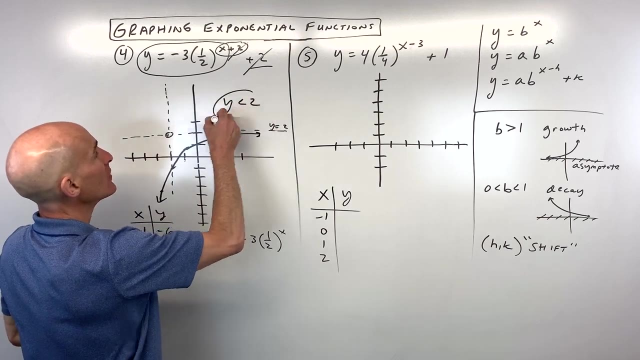 down one and a half right about there. So what you can see here is a graph. looks something like this: OK, Just a rough sketch. So the domain is all real numbers. The range is going to be: y is less than, in this case, 2.. Now, y less than 2, all the. 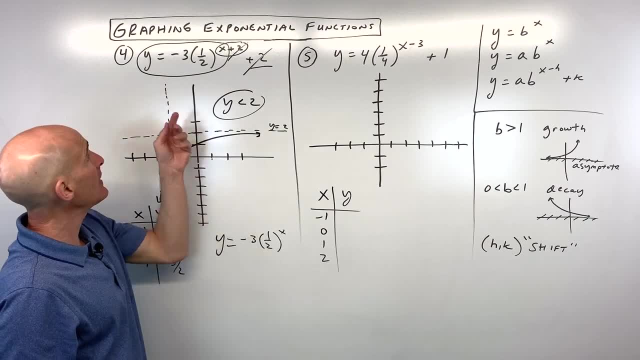 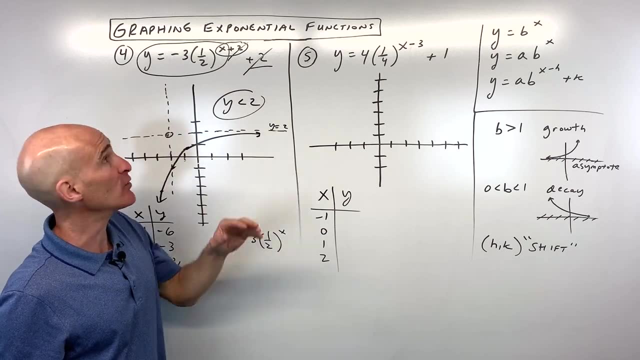 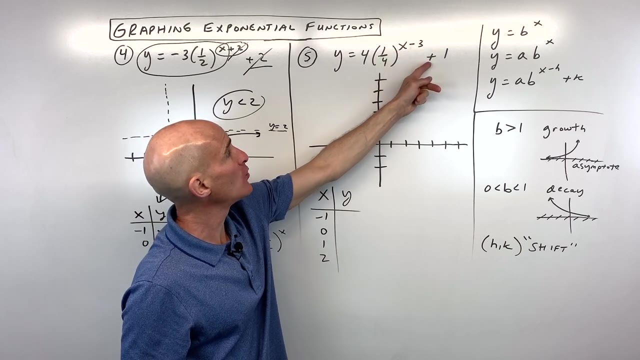 other ones we talked about so far, it was above, It was greater than, And that's because this a value was negative, So the negative reflected it over the x-axis originally, and then we shifted it. OK, So let's go to number 5.. y equals 4 times 1. fourth to the x, minus 3 plus 1.. 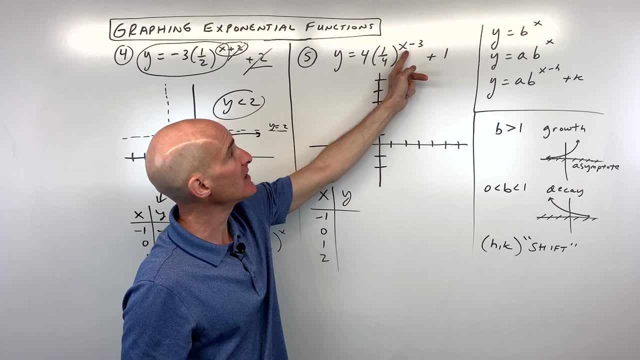 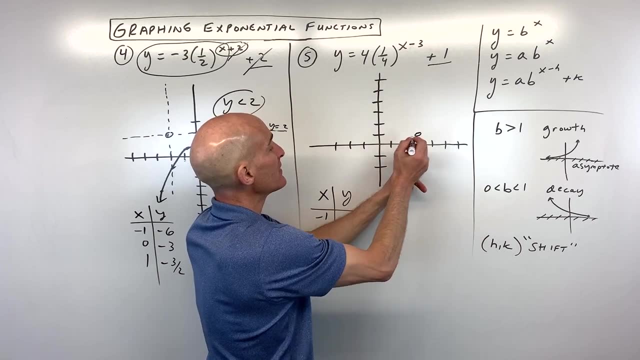 So what does this 3 do? What does this 1 do? Remember the 3,. this has the opposite effect: Minus 3 means we're actually going right 3.. This one has the same effect: Plus 1 means we're going up 1.. So we can think of that as our new starting point. I like to draw 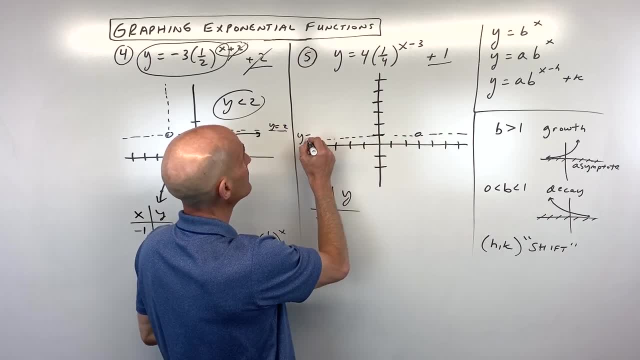 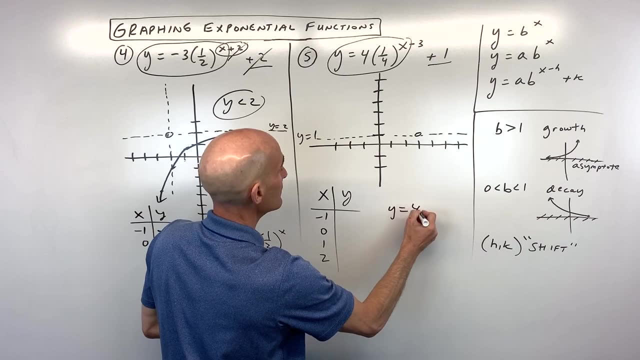 in the horizontal asymptote, This is the line: y equals 1.. And then what we're going to do is we're going to focus in on this parent function. this y equals ab to the x, And let's go ahead and make a table of values just using this parent function. Again, I like to just 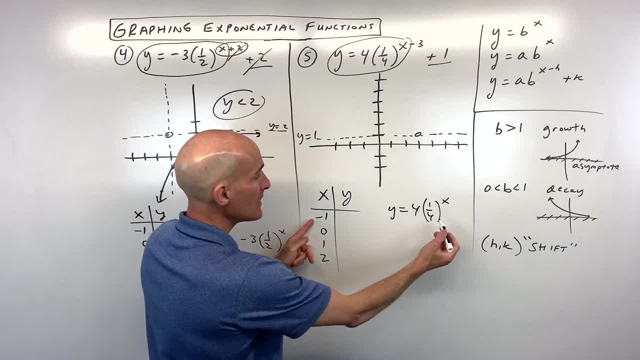 pick some simple numbers: A couple negative 0, a couple positive 1. fourth to the negative 1, that's going to be 4.. Times 4 is 6.. That's going to be 4.. That's going to be 4.. That's. 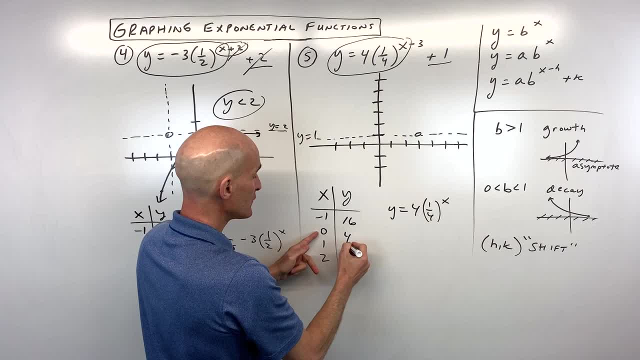 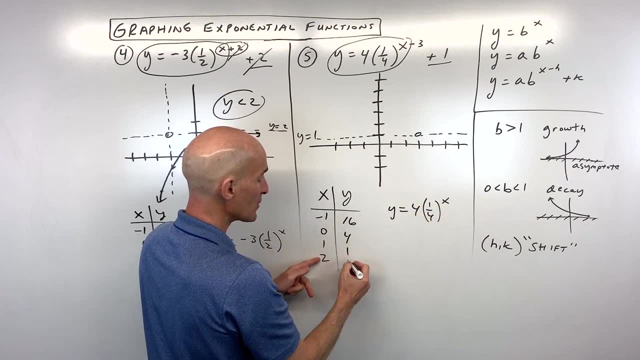 going to be 16.. 1 fourth to the 0 is 1.. Times 4 is 4.. 1 fourth to the first is 1. fourth Times 4 is 1.. And 1 fourth squared is 1. sixteenth Times 4 is 4 sixteenths, which reduces to. 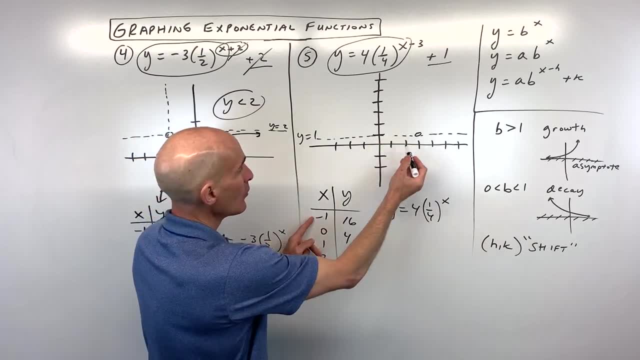 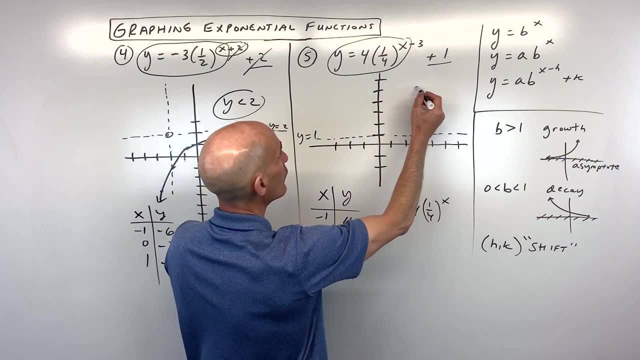